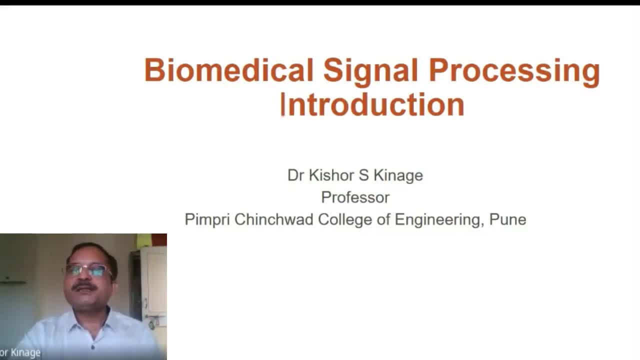 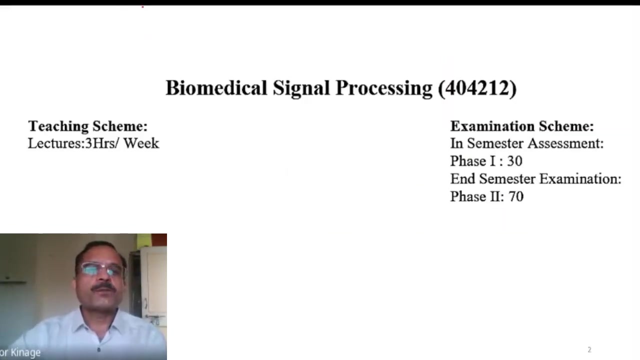 Hi. so the subject is Biomedical Signal Processing. So, as I said, today we are going to see. I will just introduce you the syllabus. Later on we will see go to the actual topics with introduction of the subject. Now you know this is as per university scheme, 3 hours of lectures per week And the assessment pattern as usual: 30 marks phase 1, 70 marks phase 2.. That is the in-SEM and the end-SEM examination. 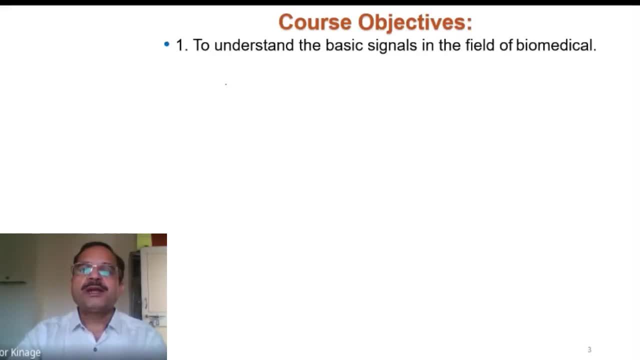 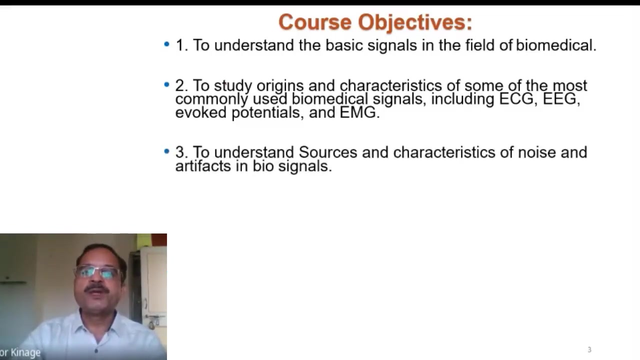 And the course objectives listed as per the university pattern. To understand the basic signals in the field of biomedical. To study origin and characteristics of some of the most commonly used biomedical signals like ECG, EEG, evoked potentials, EMG. There are more signals than this. we will see later. To understand sources and characteristics of noise and artifacts in biosignals. 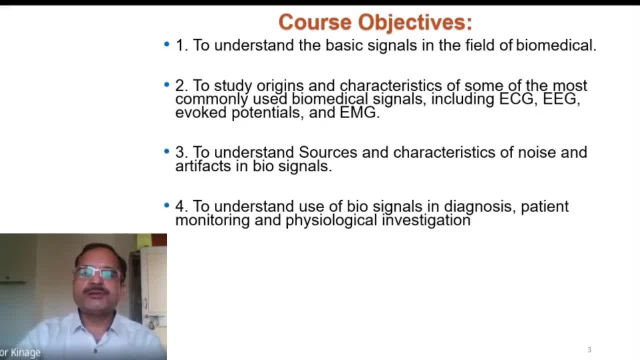 I will just read these objectives. We are going to discuss all these things: To understand use of biosignals in diagnostic, patient monitoring and physiological investigation. To explore research domain in biomedical signal processing. To explore applications of established engineering methods to complex biomedical signal problems. 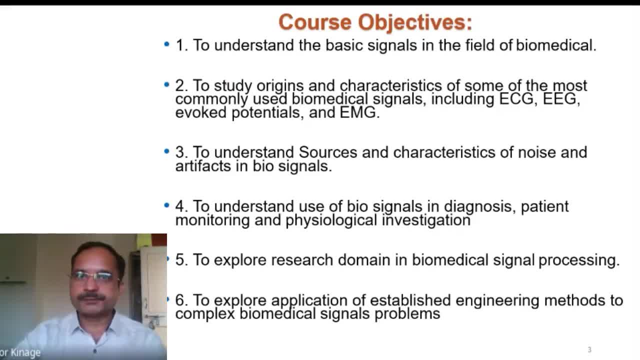 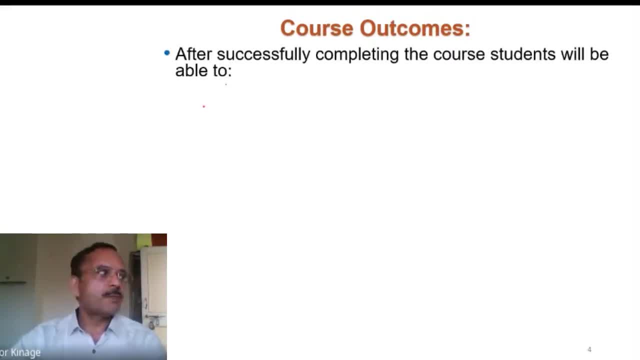 So these are the objectives as listed in the university curriculum And these are the course outcomes. So after you go through this subject, you will be able to model a biomedical system. You will be able to understand various methods of acquiring biosignals. 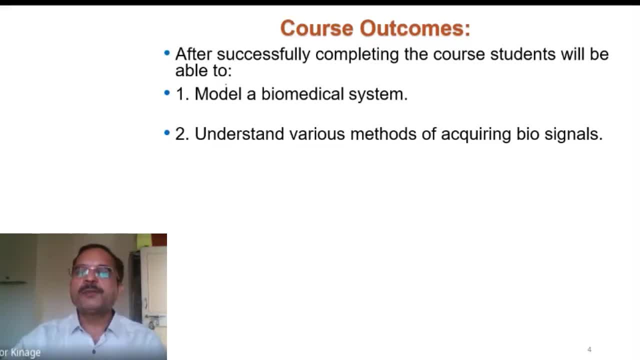 That means the different types of electrodes, where these electrodes should be placed, how they should be processed and so on. You will be able to understand various sources of biomedical, various sources of biosignals. You will be able to understand various sources of biosignal distortions and their remedies, remedial techniques. 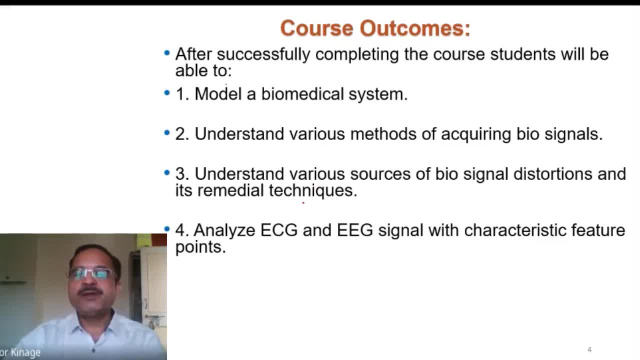 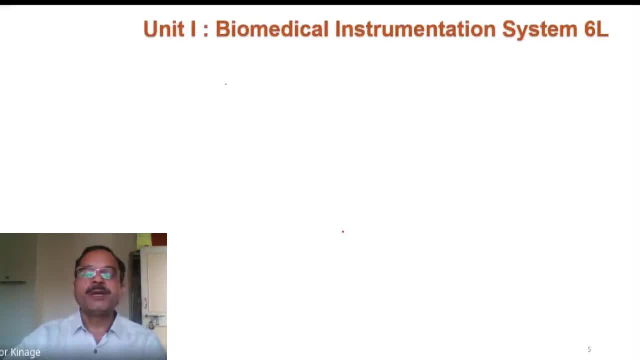 You will be able to analyze ECG and EEG signal with characteristic feature points, Have a basic understanding of diagnosing biosignals and classifying them. So these are the outcomes as listed as per the university curriculum. Now to become familiar with the syllabus, I will just go through unit by unit. 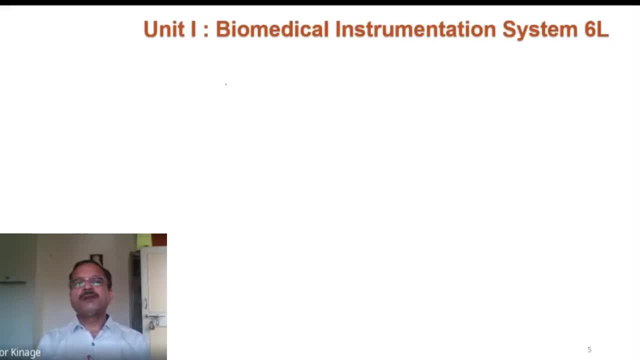 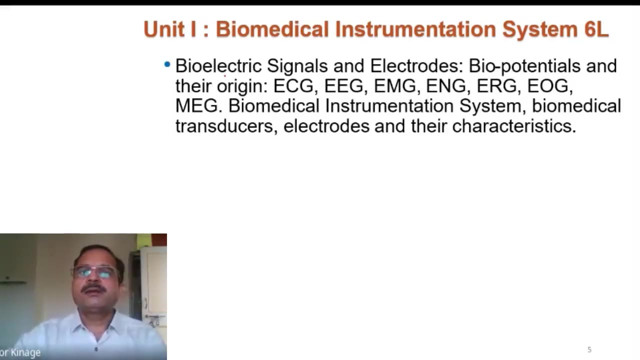 To give you the exposure to the topics which we will be covering. So the unit number one: it is about biomedical instrumentation system. So here in this unit there are actually two broader points. First one, in the first part of this unit number one we will be studying about 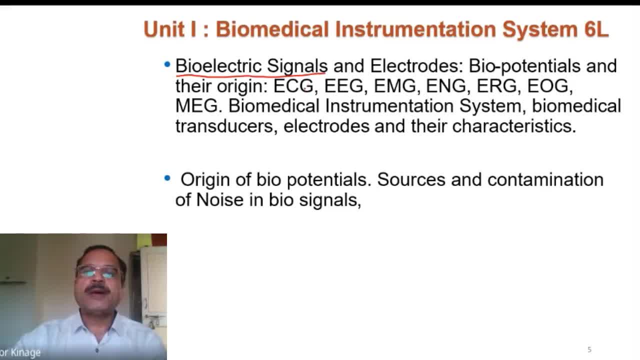 So, what are different types of bioelectric signals? Now, bioelectric signals means this, ECG, EEG and so on. Then, so actually, this ECG, EEG, these are the electrical signals Which are generated by our body. Now, what is the mechanism, how these signals are generated, what are the basic things behind that? 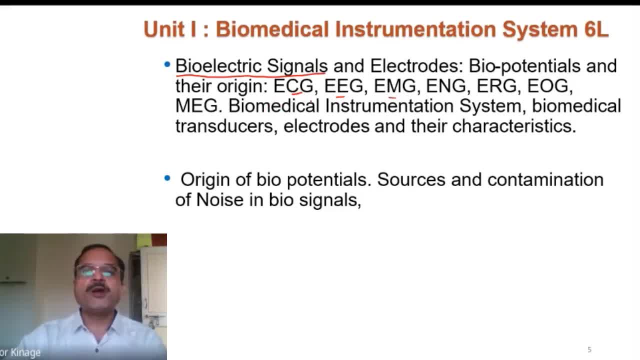 Those are called as the biopotentials, So original biopotentials. we will learn, Then we will see, in short, what are all these different types of signals- ECG, EEG, EMG and so on. Then, after that, I will introduce you the biomedical instrumentation system. 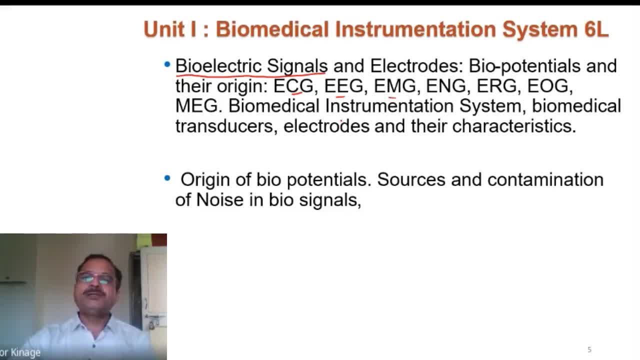 Many times this is called as man instrumentation system. So what exactly is this man instrumentation system? How it is different from our normal instrumentation system, Those things we will study here. It will be just an introductory topic. Then the types of transducers used in biomedical applications. 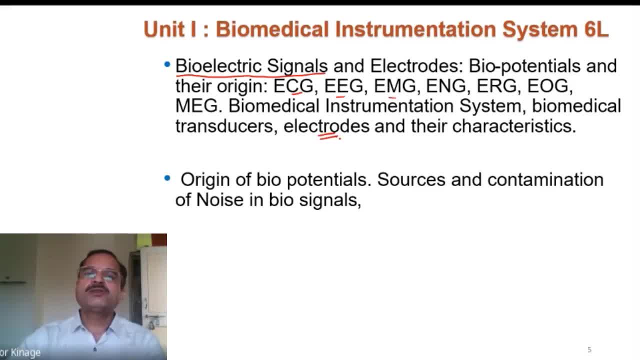 Electrodes. What are the different types of electrodes used for biomedical applications to measure all these different types of signals And their characteristics? Now, while measuring these signals, actually the magnitude of these signals, it is very small, Millivolts, sometimes maybe few microvolts also. 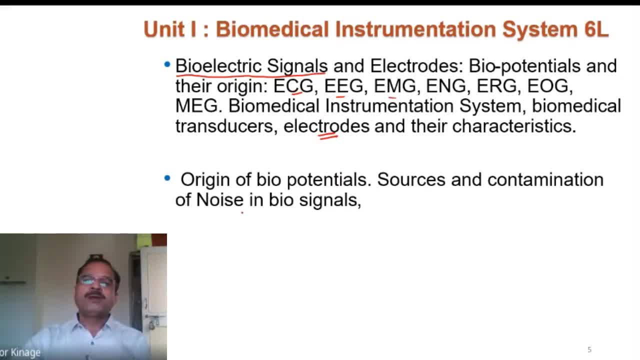 So because of that they are susceptible to noise. Then we will see what are the sources and contamination of noise in biosignals. So what are the different types of noise in these biosignals And why those types of noise occur, So that we will see here. 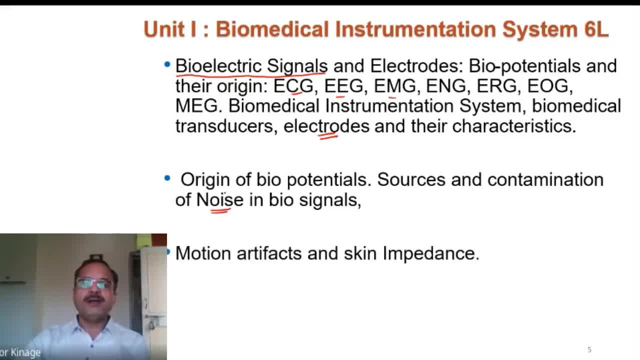 So this will be first part of unit 1. Motion artifacts and so on. So first part of unit 1. Unit 1: it will be about bioelectric signals, Then it is about the biopotentials, Then motion artifacts and skin impediments. 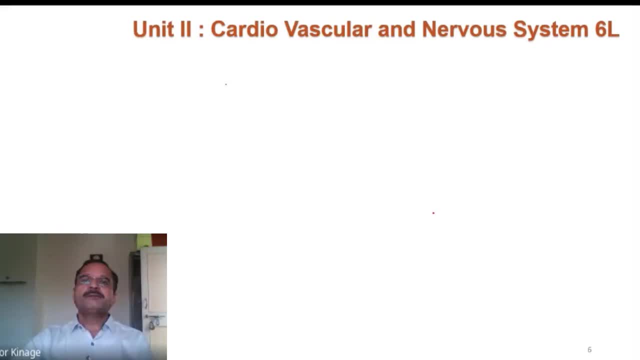 So this is our unit number 1.. Then, in unit number 2., We will study cardiovascular and nervous system. Now the terminologies you might have heard This: Cardio means it is related to heart, Okay- And nervous system, it is about a brain and all different types of network of nerves existing in our body. 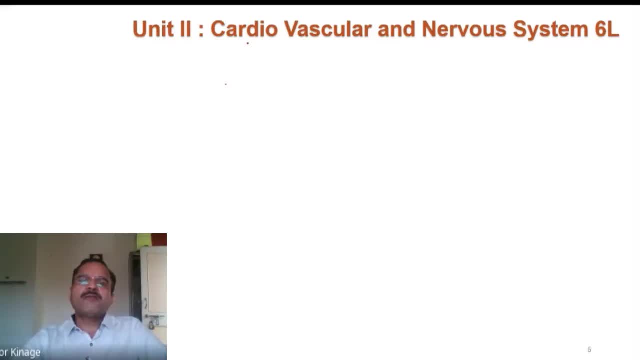 Now, both these systems are very important. Cardiovascular, it is the system related to heart. And nervous system, it is related to the brain signals And the various nerves Which are being distributed throughout our body. Now this system generates some electrical signals. Okay, 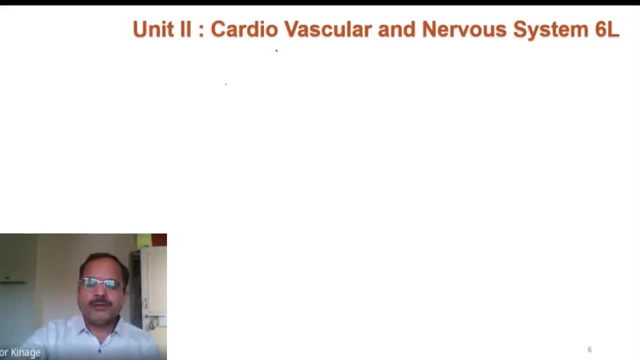 So what are those? Now, before going to, Before studying this- electrical signals generated by cardiovascular system And the nervous system. You should know How actually our heart works. What is the basic principle? How our heart works, How our nervous system works. 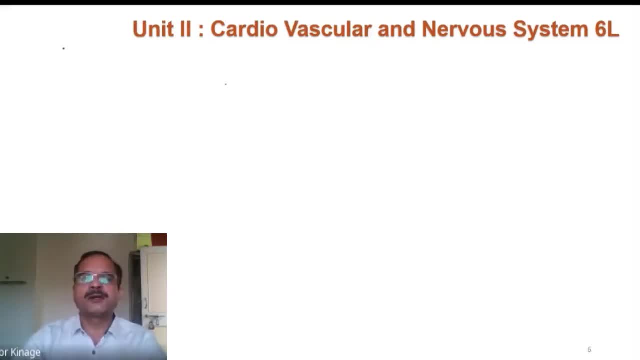 And how it actually produces some electrical signal. So actually our subject is biomedical signal processing, But that means how to process biomedical signals. But before processing the biomedical signals You should know what is the origin of these signals And how these signals are produced. 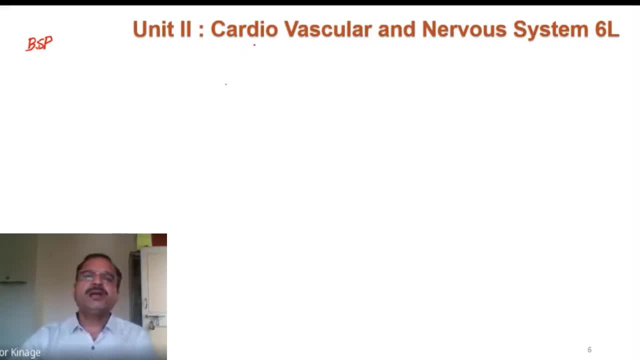 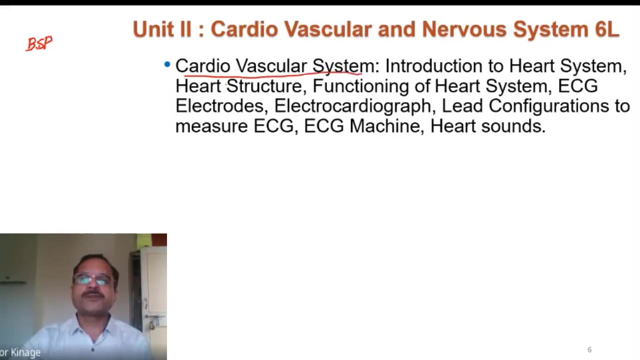 Right. So that's why it is necessary to know the basic working of cardiovascular system and nervous system. So unit number two it is about this. So there are two parts in unit number two. First part it is the cardiovascular system, So introduction to the heart system. 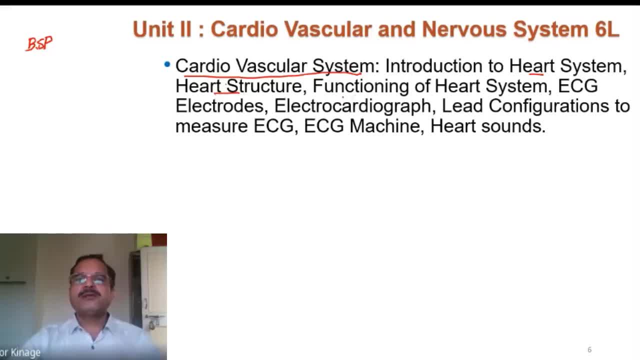 What is the heart structure, What are the How the pumping action takes place in the heart, What are different types of valves, Right, The different types of arteries, Then how the heart functions. So what is the pumping action taking place done by the heart? 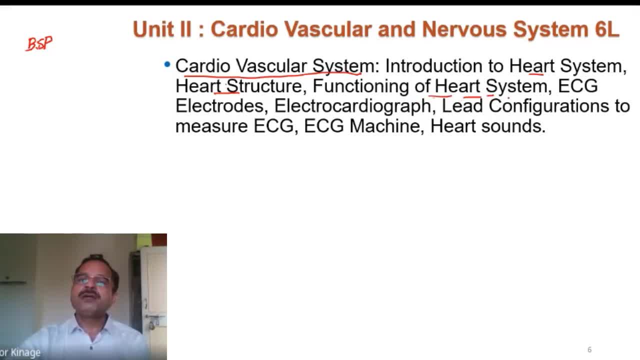 And the electrical signals generated by the heart, How the electric signals are generated And what are the corresponding graphs for that. We call it as ECG Electrocardiograph, The electrical signals generated by heart muscles called as electrocardiograph. 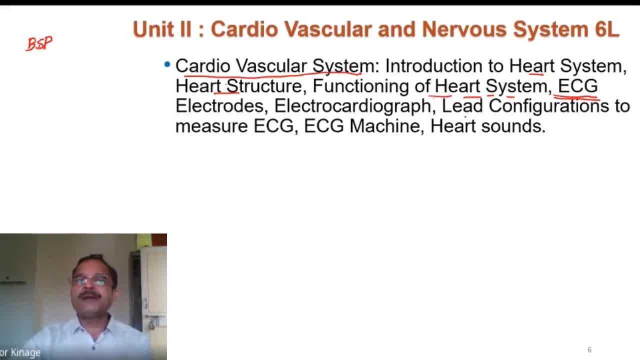 Okay, Now then, what are the lead configurations to measure ECG? Lead configuration means, Lead means these are the terminals, The wires. So how these wires are connected, What type of electrodes are used to measure this ECG signal Which is finally given to some ECG machine? 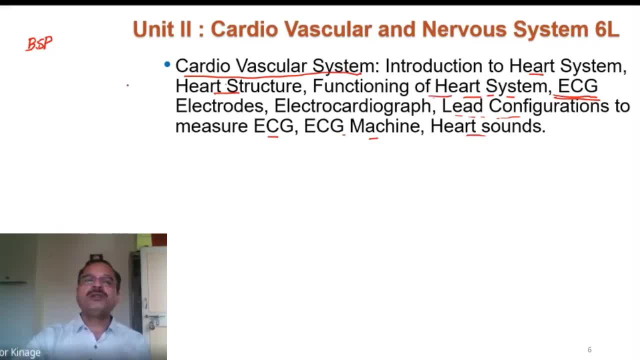 And what are heart sounds. So all these things we are going to learn in this first part of unit number two, That is, cardiovascular system. Now in the next part of unit number two We will be learning about nervous system. So here We will see. 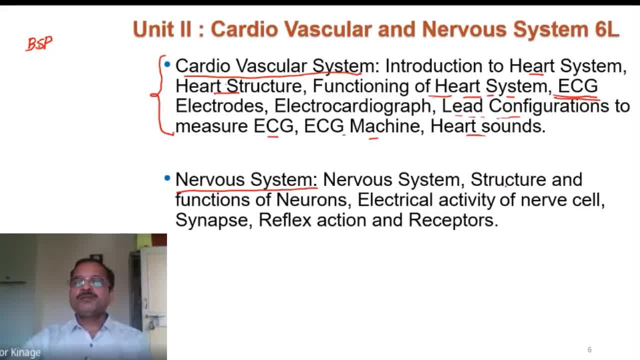 The basic functioning of nervous system. What is the structure and functions of neurons And electrical activity of nerve cell, So how these nerve cells produces electrical signals. So what is synapse? reflex action receptors. So this is our second part of unit number two. 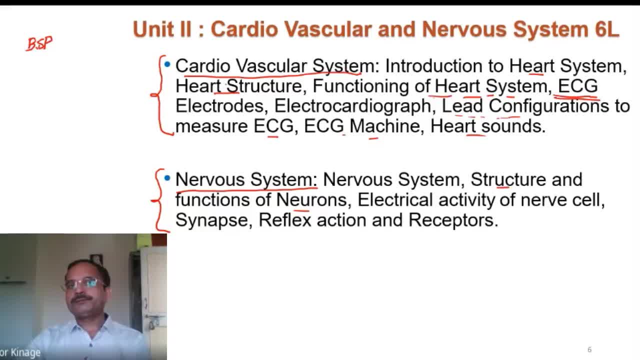 That is nervous system. So unit number two, As we have discussed It, is the introduction of how our heart works, How the electrical signals are generated by our heart And nervous system. What is the functioning of nervous system And what are the? 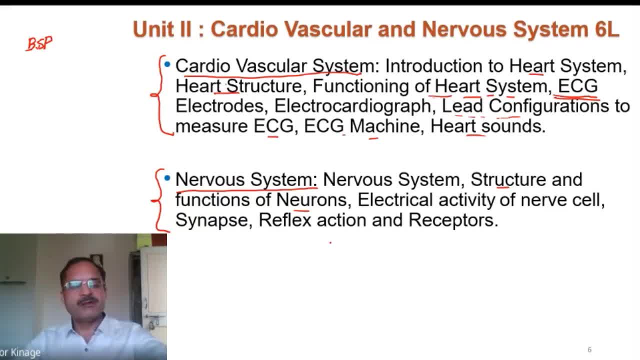 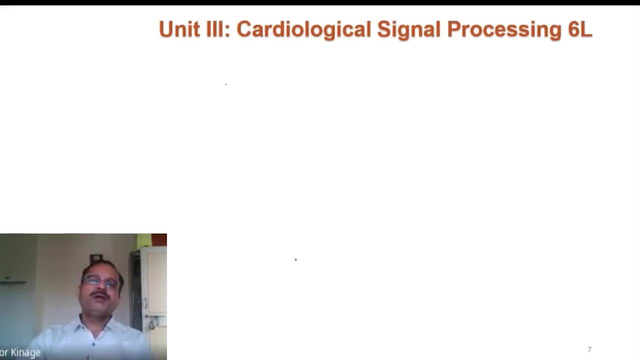 How the electrical signals are generated by our nervous system And how they are measured. Okay, So that is This unit number two. Then, after studying unit number one and two, Then we will proceed to actual signal processing. Okay, So unit number three. 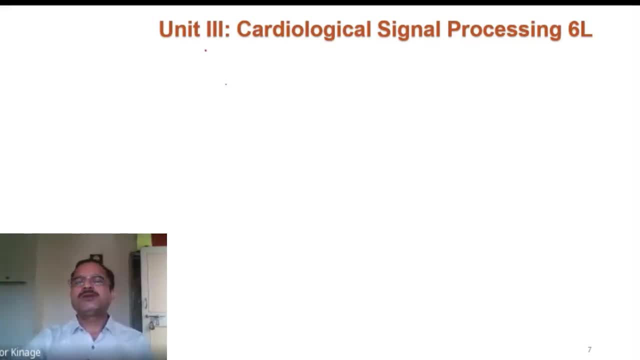 It is about cardiological signal processing. Now, in unit number two, We will be studying the basic functioning of our heart, How the pumping action takes place, How the electrical signals are generated. We call it as ECG, That is, electrocardiograph. 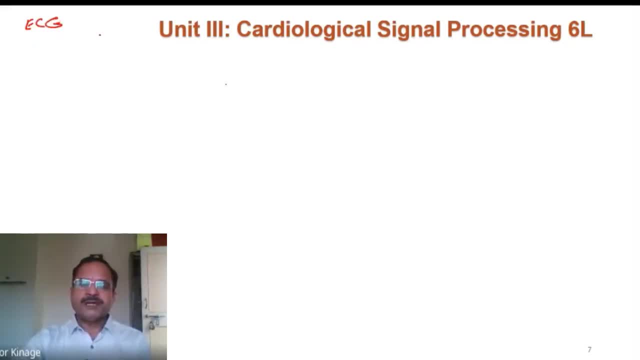 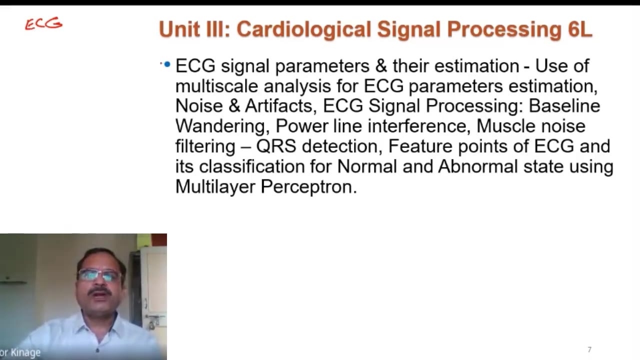 Right Now in this unit We will see what are the characteristics of ECG, How this waveform of ECG looks like And the processing The signal. See how this, What type of information this ECG signal contains And the corresponding processing of this ECG signal. 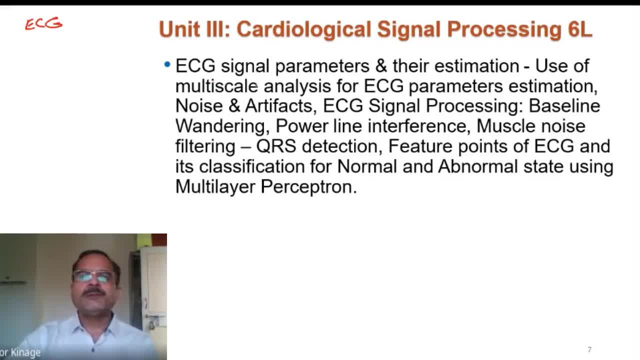 So that we will see here. So The points are like this: ECG signal parameters And their estimation, Use of multi-scale analysis for ECG parameters. estimation, Noise artifacts, ECG signal processing Baseline, wandering Power line interference. 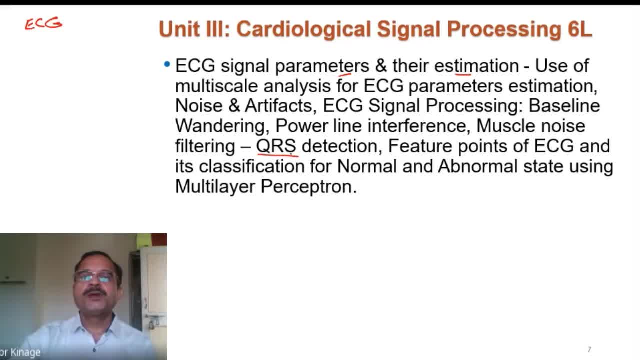 Muscle noise filtering. QRS detection: This ECG Waveform It has. It is classified, It is divided into different parts, So QRS. These are the parts of this ECG signal. So how Q wave is detected. 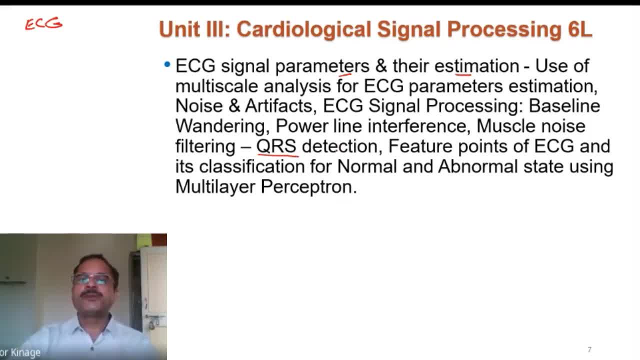 R wave detection, S wave detection And so on. So that is called as QRS detection, Then picture points of ECG And its classification of normal For normal and abnormal state Using multi-layer perceptron. So So ECG is ECG signal. 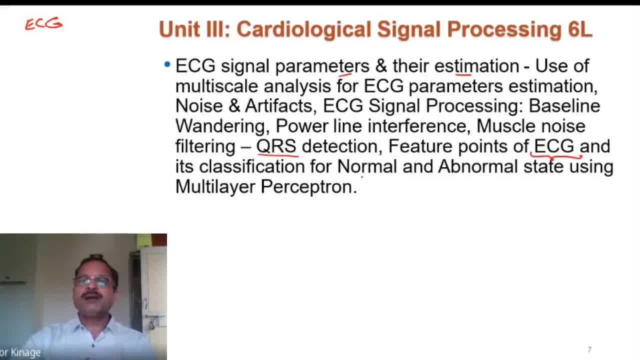 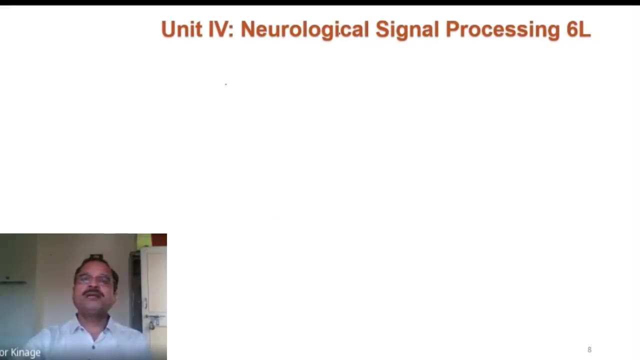 When it is recorded, How to classify Whether it is a normal ECG Or there is some abnormality in that, So that we will find out using multi-layer Perceptron. So this is about cardiological signal processing. unit number four, it is about neurological signal processing. so in 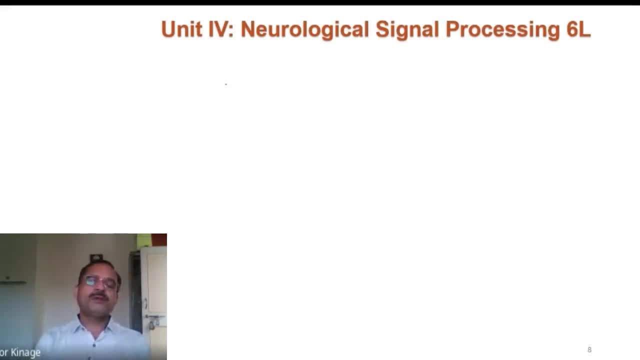 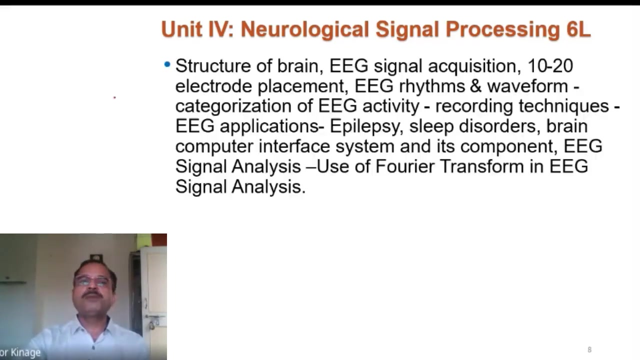 unit number two we will be studying the basic working of the our nervous system, how our brain and all the nerves inside our body, how the electrical signals are processed, how the electrical signals are generated and what are the characteristics. okay, so in unit number four it will be about the processing of 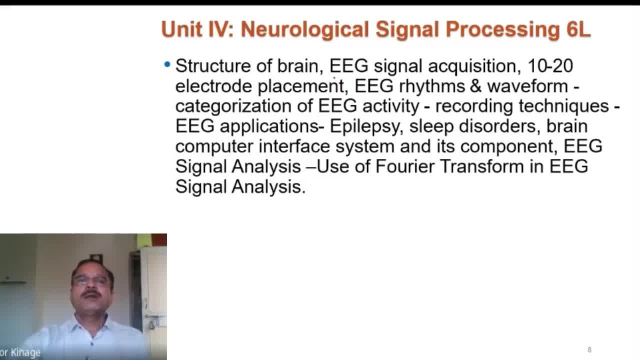 neurological signal, so the signal generated by our neurological system. it is called as EEG electroencephalograph. okay, so we'll see what is the structure of the brain, how, how the signal, that means how the EEG electroencephalograph signal it is acquired. now, to acquire this signal we'll have to place 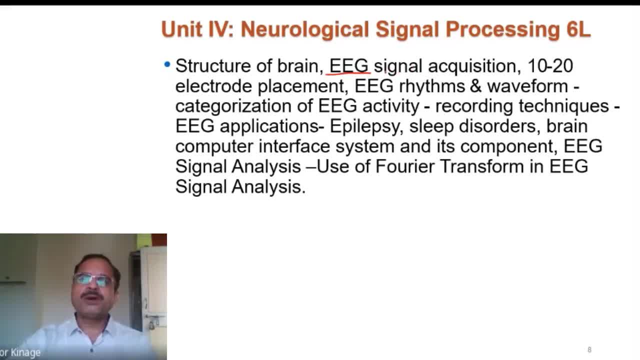 different number of electrodes on our brain right. so what is the system or what are the techniques to place the electrodes? so it is called as ten: 20 electrode placement and 20 electrode placement. so this is actually the technique where, how to place the electrodes to measure this EEG signal at. 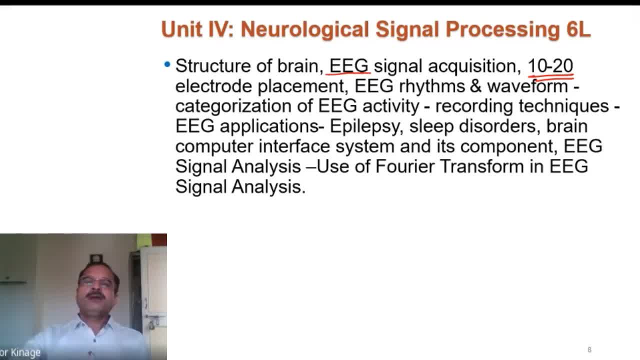 what are the corresponding locations then? which method is used to place the electrodes in brain, The characteristics of this EEG, how it varies as a signal, So EEG rhythms and the waveform Categorization of EEG activity. and the recording techniques and applications. Applications of EEG. 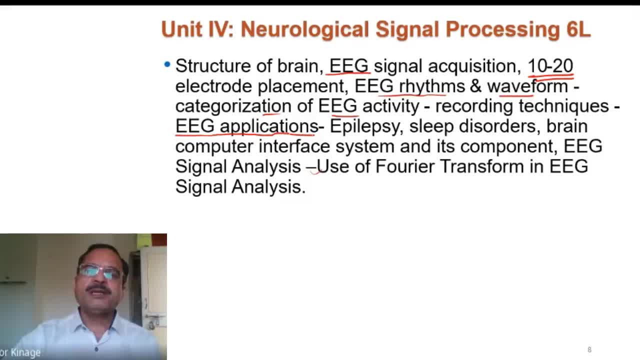 So from this EEG signal, if you process this, the outcome of this EEG signal processing, you can conclude many things. What are the abnormalities in our brain, normal functioning of our brains, or are there any disorders like epilepsy, sleep disorders? So these type of disorders can be predicted? 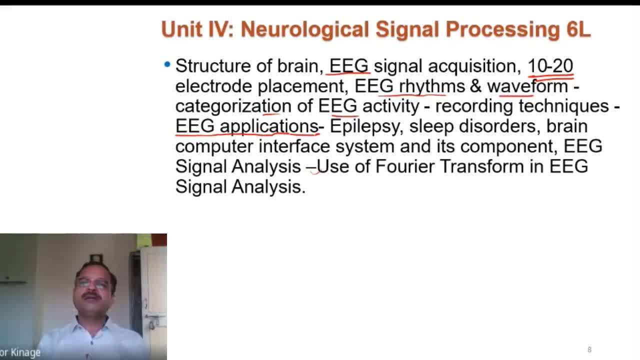 So we can be predicted by processing this EEG signals. Then what is the brain-computer interface system and its component, How to interface the computer with our brain? Then EEG signal analysis will be using Fourier transform to analyze the EEG signal. So how to use Fourier transform for analysis of EEG signal? 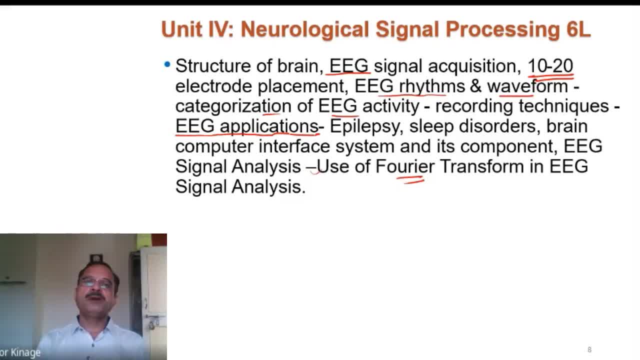 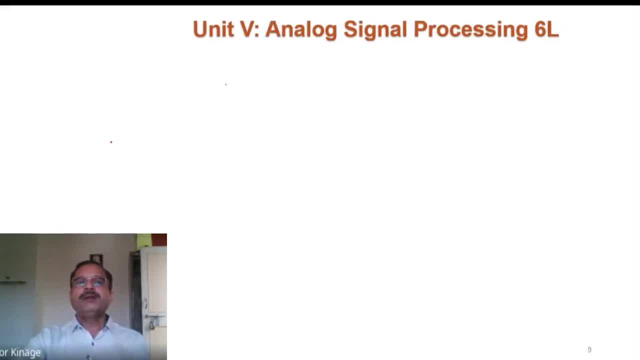 So all these things will be discussed, So all these things will be studied here. Unit number 4, that is neurological signal processing. Then next one, unit number 5, it is analog signal processing. So here now in unit number 3 and 4, as we have seen, it is unit number 3, it is specifically devoted to cardiovascular system. 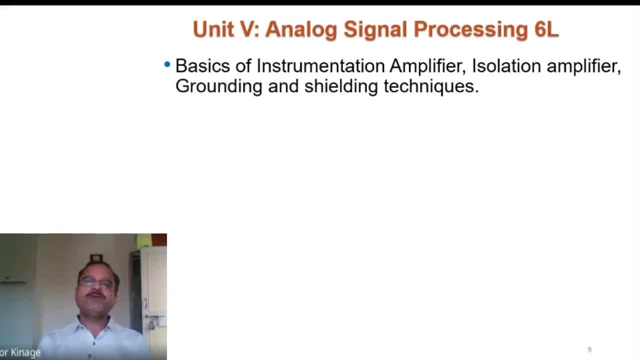 That means the ECG, ECG signal And unit number 4, it is devoted for EEG signal, That means the signal related to brain. Actually, apart from this EEG and ECG, there are many more electrical signals which are generated by our body. 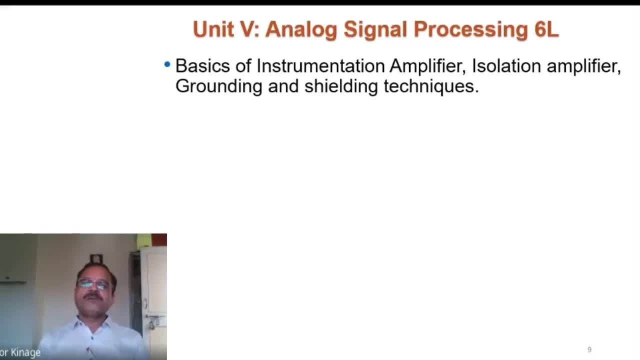 For example, for our eye we have EEG, electro-oculograph, EOG. That is EOG, Electro-oculograph oculograph- the signals generated by our eyes, Then our body muscles generate signals, So that signal is called as EMG, electromyograph. So like this: there are different types of 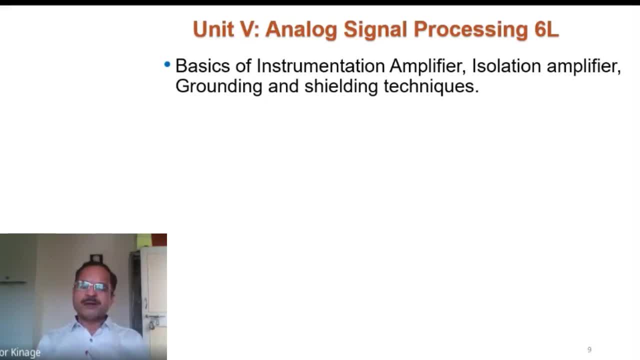 signals actually generated by our organs. But in our syllabus we will be focusing mainly about ECG and EEG. That means the brain signals and the heart signals. Okay, So that was our unit number 3 and unit number 4.. Now, in unit number 5, we will discuss about the analog. 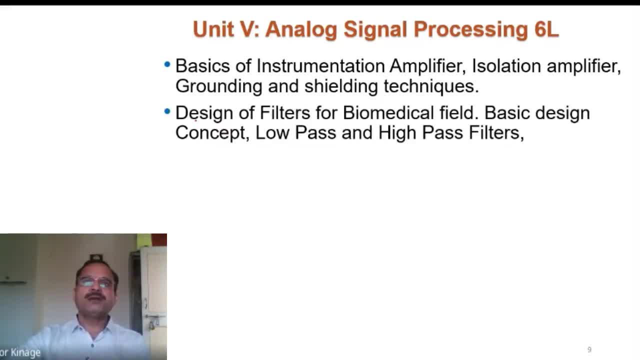 signal processing required to process this biomedical signals. So here we will see what are the basics of instrumentation: amplifiers, Isolation amplifiers which are useful for biomedical equipments, grounding techniques, shielding techniques, these things. Then design of filters for biomedical field: Basic design. 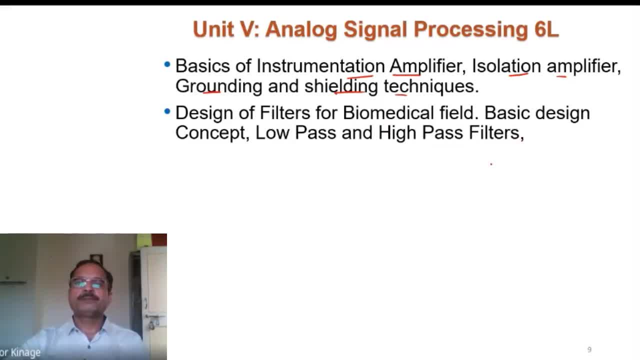 concept low pass and high pass filters, So bat pass filters, band stop filters, band reject filters. So all these, the fundamentals of all these filters you might have studied in digital signal processing. So here we will study how to use this filters to in case. 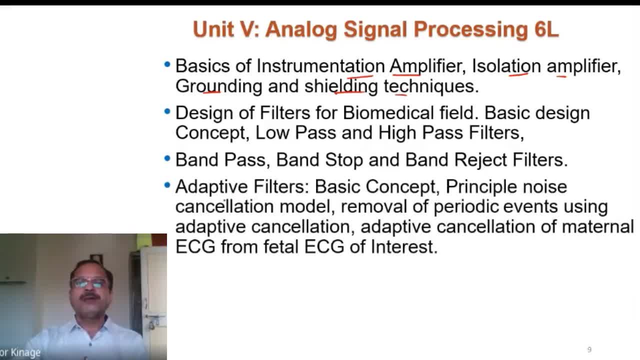 of biomedical signal processing. Okay, Then, in the later part of this unit- number 5,, we will study adaptive filters. What is the basic concept of adaptive filters? Principle of noise cancellation, model, Removal of periodic events using adaptive cancellation, Then, essentially, 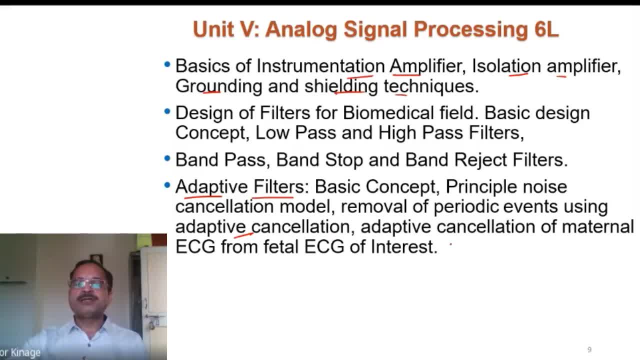 we will see of this unit 5, which is stage 1.. This unit 5, the basic concept of adaptive filters, And then stage 2, the basic concept of noise cancellation model. This is the basic. Then add up to cancellation of maternal EEG, ECG from fetal ECG. This is one actual application of how this signal processing can be applied for real time applications. 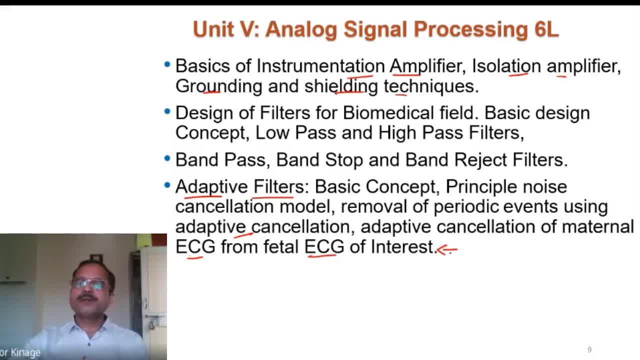 So what this means is that during pregnancy, the fetal, the child, when this ECG is measured from the heart of the mother, it will consist of heart signals produced by the fetus. That means the fetus, That means the child. Now, by measuring that ECG, we can apply some signal processing techniques and we can separate the maternal ECG from the fetal ECG. 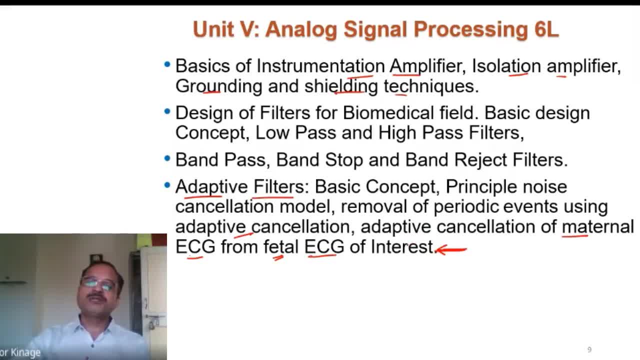 So that is actually one of the real time applications of how this signal processing can be applied. So this is what is analog signal processing- Analog things we have studied in the earlier semesters, So we will see here how these things can be applied for in case of biomedical signals. 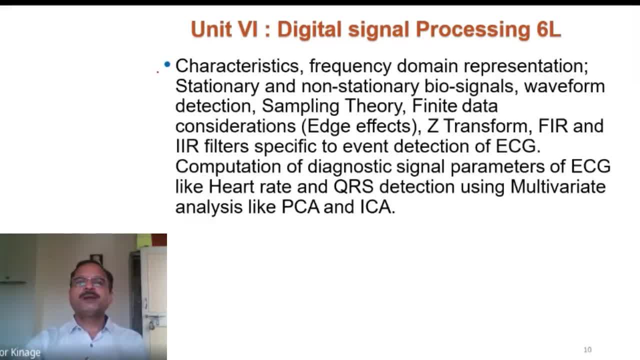 Then digital signal processing. So the digital signal processing that means all this: frequency domain representation, stationary, non-stationary biosignals, waveform detection, sampling theory and so on, FIR filters, IR filters. how to apply all this digital signal processing techniques in case of biomedical signals? 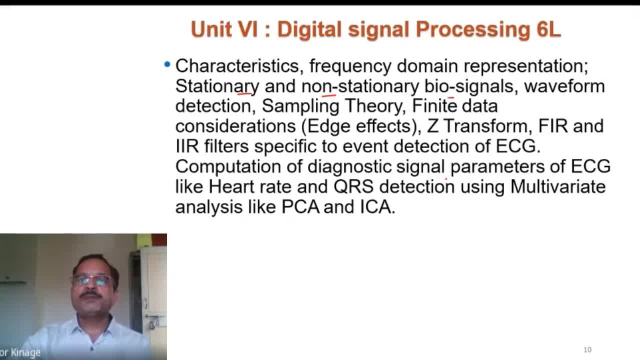 So that we will study here in short Computation of diagnostic signal parameters of ECG, like heart rate and QRS detection, using multivariate analysis like PCA and ICA. So how to use PCA? PCA, that is principal component analysis. ICA, that means the independent component analysis for heart rate and QRS detection. 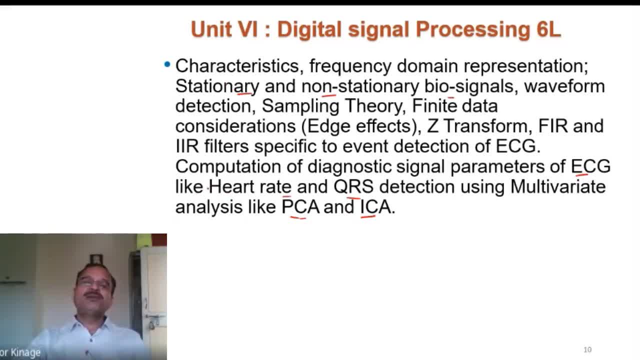 So that we will study here. So actually whatever subject you have studied- digital signal processing. So in unit number 5, we will see how to apply all those concepts to process biomedical signals. So this is our unit number 6.. Okay, 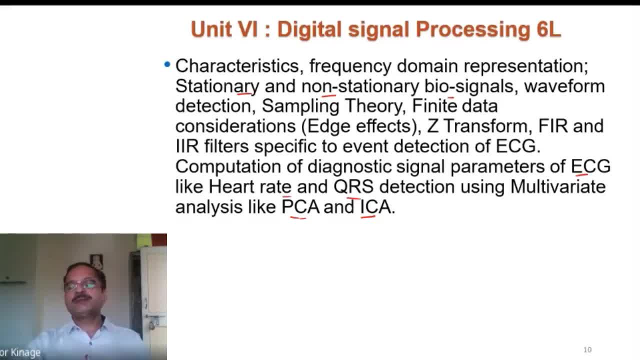 So this was about the syllabus, All the 6 units. So first two units. it is about the first unit. it is the introduction to biomedical signal processing, the instrumentation system. Second unit: it is about the cardiovascular system and the nervous system. 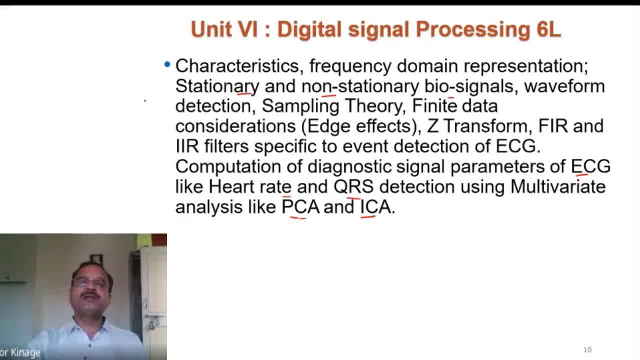 Third unit: we have seen the processing of cardiovascular signals. Fourth unit: it is about the nervous system, functioning of nervous system and how the nervous system signals are produced. Then unit number 5, it was about analog signal processing: How to use analog signal processing concepts to process biomedical signals. 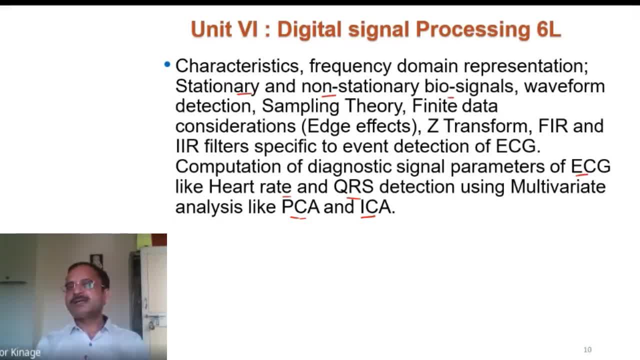 Then unit number 6, DSP, that is, digital signal processing, All the subject, what you have studied till now, digital signal processing, How to apply those concepts for biomedical signals. So these are the 6 units we will be learning here. It is a very interesting subject, practical point of view, practically to apply for some projects like that. 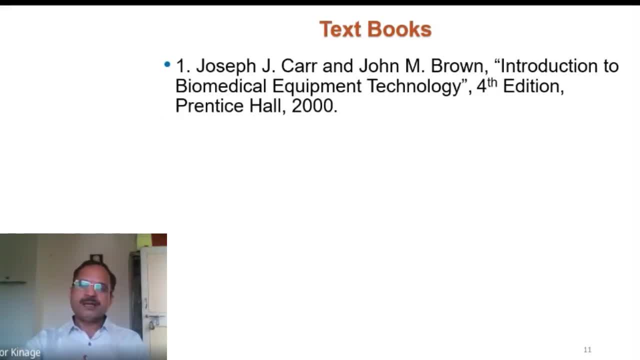 Now the books I am listing here. These are the books which are prescribed as per unit number. Now, apart from this, you will find many more books available. So first one by Joseph Carr and John Brown: Introduction to Biomedical Equipment Technology, published by PHI. 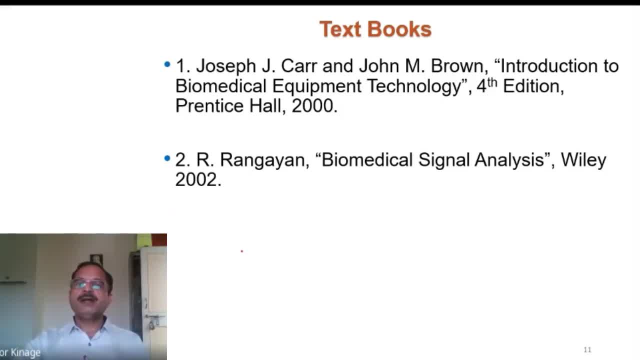 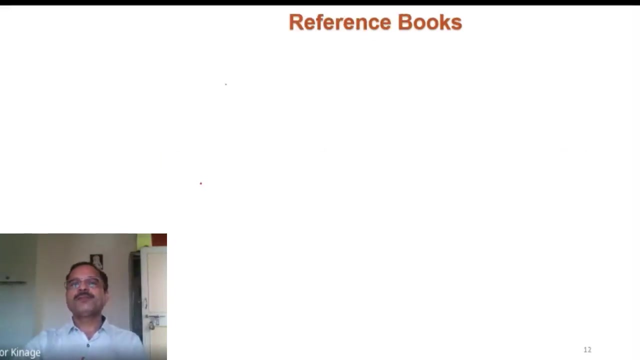 Second one, it is by Rangayan, Biomedical Signal Analysis. The third one, Biomedical Signal and Biomedical Image Processing. So these are the textbooks prescribed by Mumbai University, sorry textbooks, sorry, prescribed by Pune University. Then the reference books: Khandpur, Handbook of Biomedical Instrumentation. 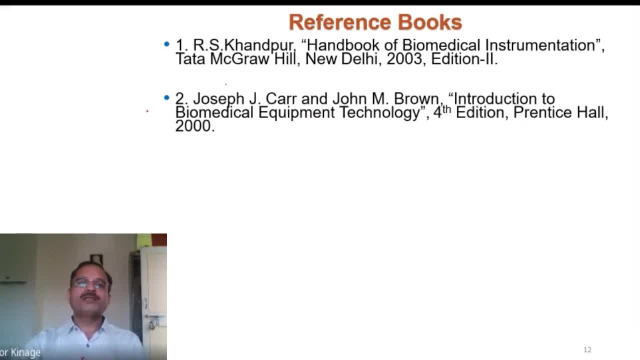 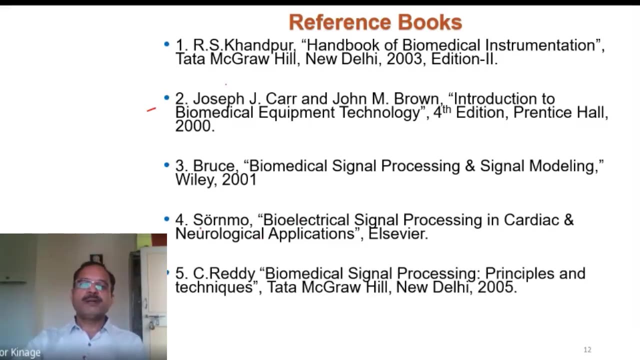 This they have repeated, actually reference book as well as textbook. Then third one by Bruce: Biomedical Signal Processing and Signal Modeling, Bioelectrical Signal Processing and Cardiac and Neurological Applications, That is by Somu. Then fifth book by C Reddy, Biomedical Signal Processing: Principles and Techniques, by Tata Meghalaya. 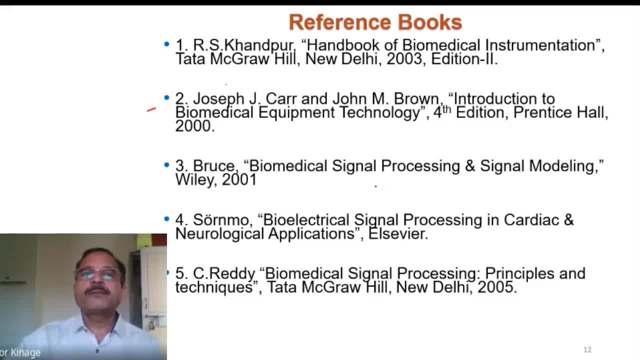 The first book by Khandpur for unit number 1, to begin the subject, you can start with this book by Khandpur. This is actually an instrumentation book, But our subject, it is mostly about signal processing, biomedical signal processing. 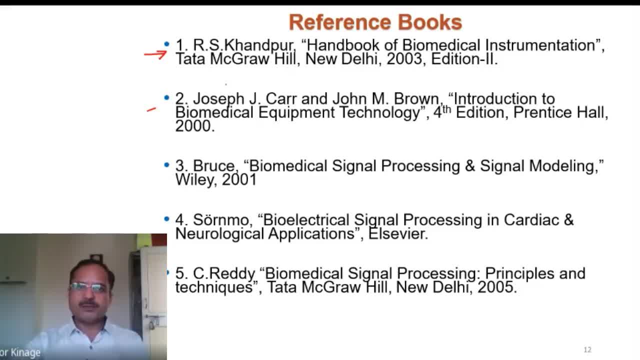 But for unit number 1, you can refer this book, the first one. For other units the other books will be useful And time to time you can refer this book And time to time I will tell you the type of books to be referred for the actual topic. 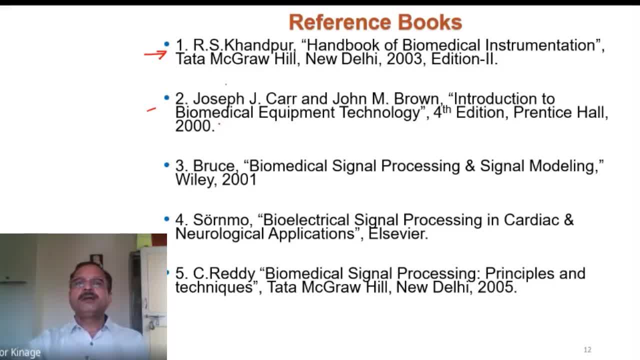 when we will cover those topics. So this is about the introduction to the subject, The content, what we will be studying here, Textbooks and the reference books. The last one, it is by Tompkins, Biomedical Signal Processing. Okay, 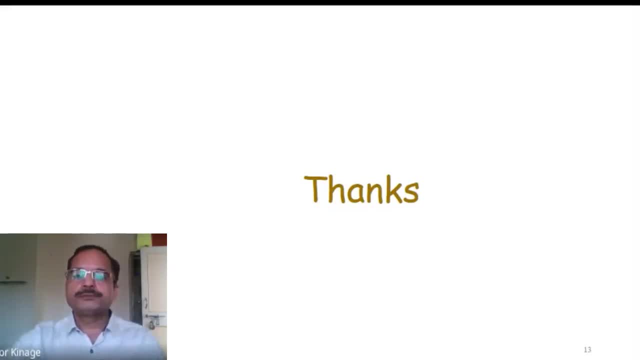 Now again over to you. Okay, Now, if there are any queries from you related to the subject or, in general, any queries how to study this subject or the material and so on, we will discuss for few minutes And after that we will wind up. 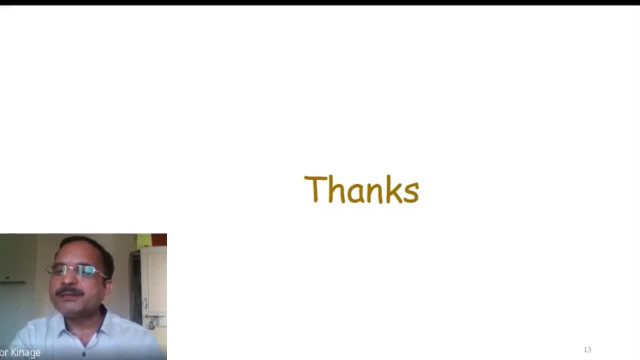 Now, earlier at the beginning of this lecture, I asked you some question. What is the reason for selecting this subject? Biomedical Signal Processing- Somebody? yeah, Dipali Kale has typed her reply in the chat box. I will just read it. 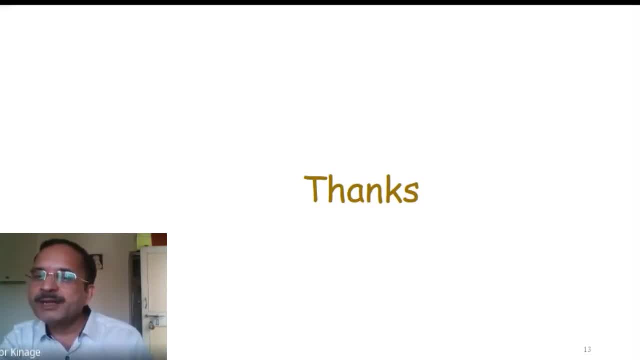 Health is most important part of our life, And this subject teaches me how, how to we can connect electronics with. we can connect electronics with biology. That's why I chose this subject. Yes, correct, So actually in our four years of engineering. 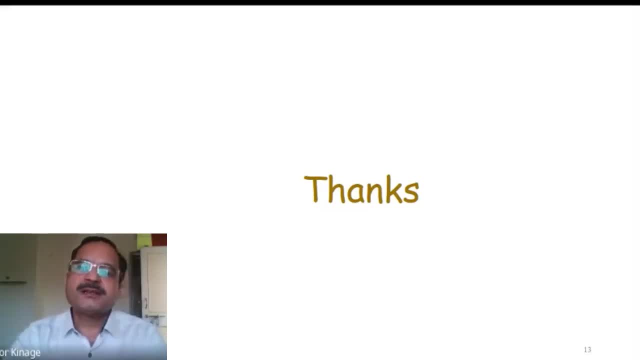 first year and second year we just learn very fundamental subjects. Okay. Then third year onwards we start a little bit applications And the more application-oriented subjects actually begin, begin introduce. more application-oriented subjects are introduced in the final year, But it is again just the introduction. 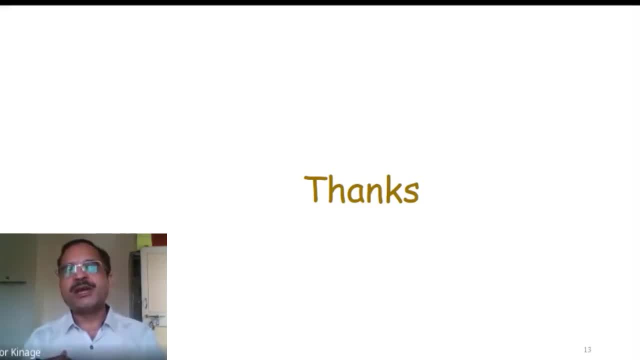 So the actual field it is actually after graduation, After you complete your B. then you will come to know that I have just learnt the little little part of everything, And later on you have to develop yourself, you have to choose your area of interest. 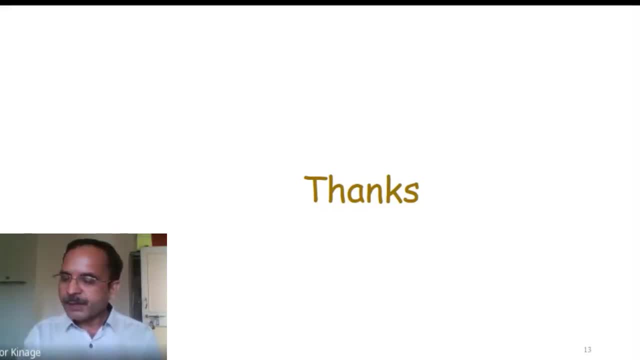 and start working Now. the various areas of interest are the different fields related to electronics. One of that it is biomedical engineering, So in the next lecture I will discuss more about this. So biomedical engineering, that means actually when we study our 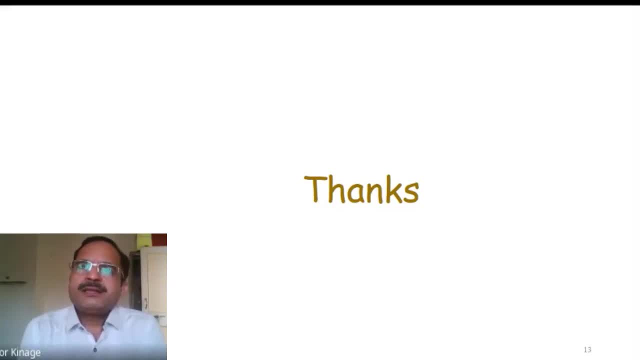 see why we are actually. this is just you can say: this is a medical thing, right, Medical, but nowadays, each and for each and every purpose, medical diagnosis, even for treatments and for surgical, for surgery, operations and so on.